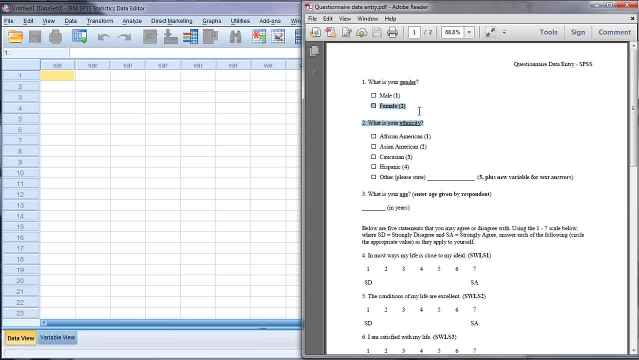 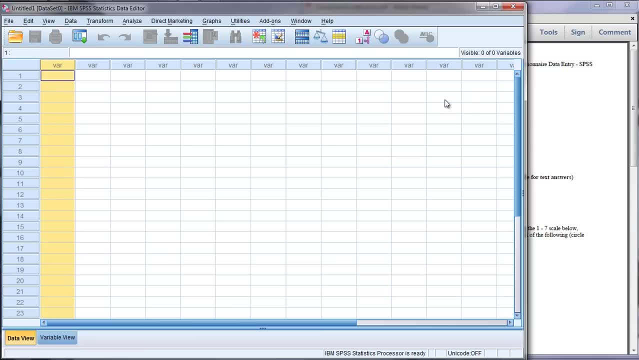 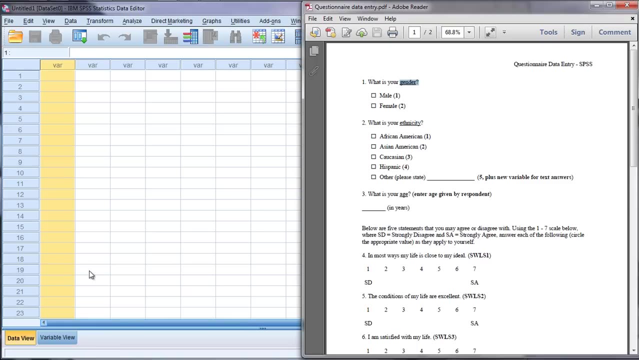 every time we have a possible answer such as male or female, we need to create a variable in SPSS that will hold those different answers. So our first variable needs to be gender, and that's why that's underlined there, just to assist us as we're doing this. So we want to make sure we're in the variable. 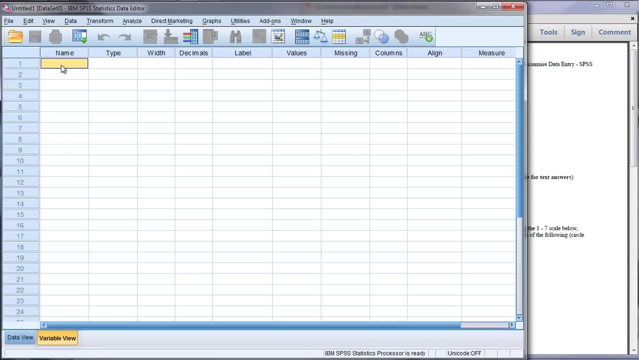 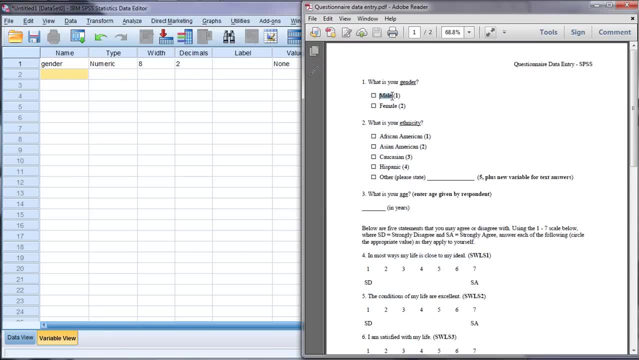 view tab And then in the first row here under name, we want to type gender and then press enter And that creates the variable gender. Now notice, here I have two options: male and female. So when people respond or circle or check here that they're a male. 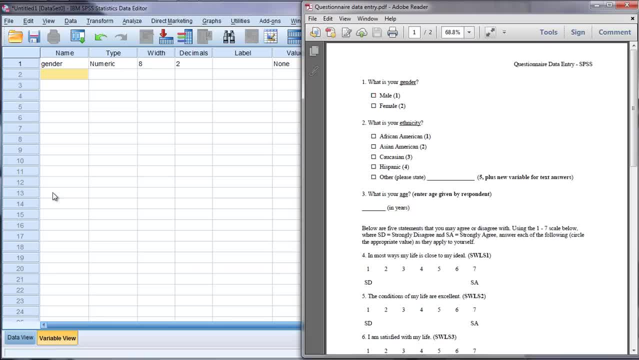 I need to enter into SPSS some number to indicate that. So we always want to enter numbers whenever possible in SPSS because SPSS, for the vast majority of analyses, performs statistical analyses on numbers, not on words. So I wouldn't want to enter male, female and so forth. 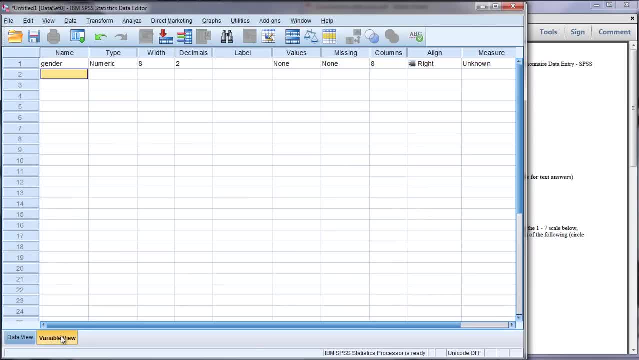 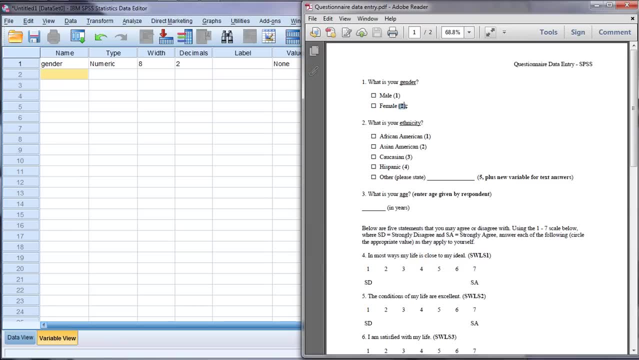 I want to enter ones twos, and so on. So notice here. I just arbitrarily decided males get a one and females get a two. It could have been the other way around, but since male was the first name listed, I went ahead and gave that a one and then. 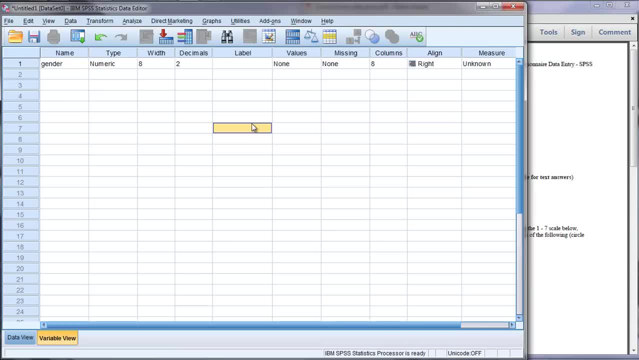 for females, I gave it a two. So what we want to do in our data file here is go ahead and go to values this column. click on the none cell, Notice these three dots appear. They're called an ellipsis. Click on that and then our first value notice. 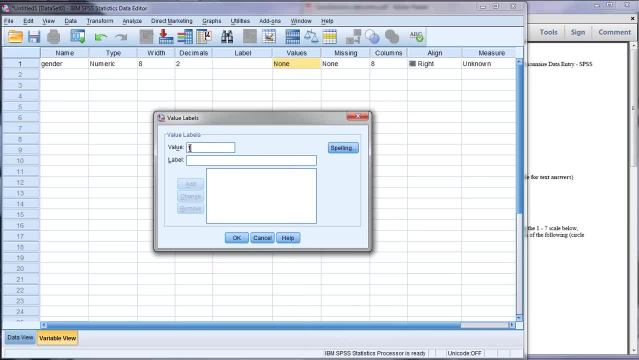 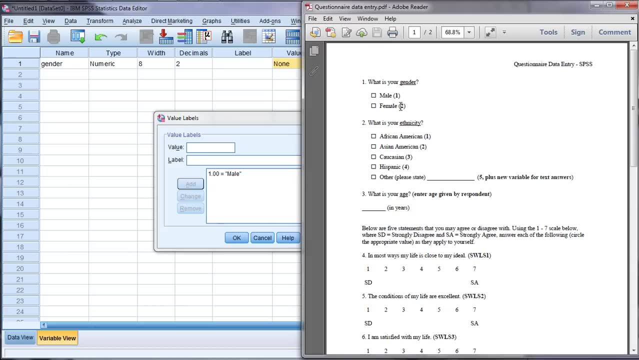 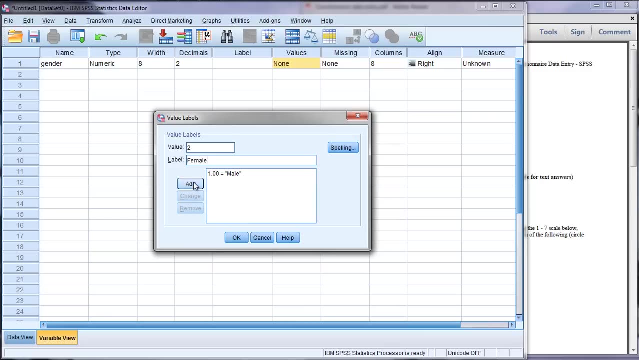 here one is male, So value of one and then type label male and then click Add, And then our second value of two is for females. So go ahead and enter a two for value and then female, click Add and then we're done with that. You want to see? 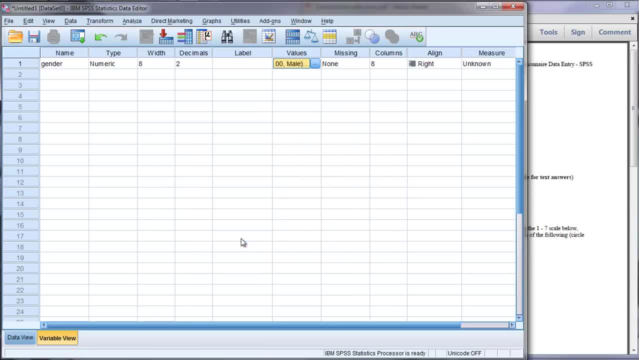 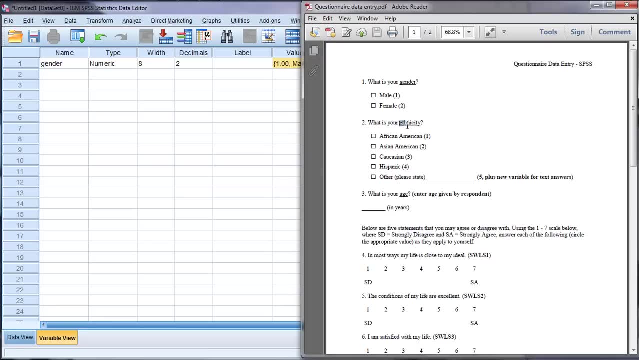 both of them down here and that looks good, So click OK. Now those labels are in here and I'll show you how that works when we enter some numbers in a minute. Ok, next we have ethnicity, So I'm going to call this variable ethnicity, So go. 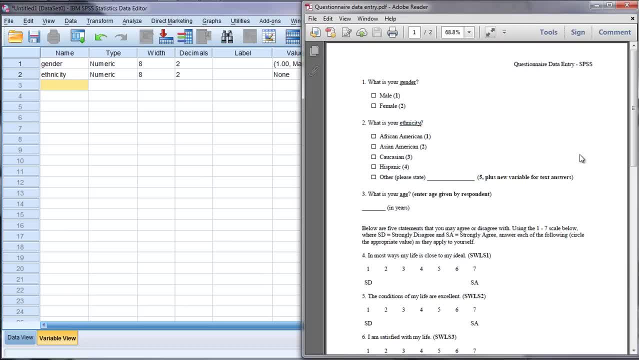 ahead and type that in Press Enter. And then we're going to do the same thing. We're going to create value labels here. So one is African-American, two is Asian-American, and so on, And I'll just do that very quickly.